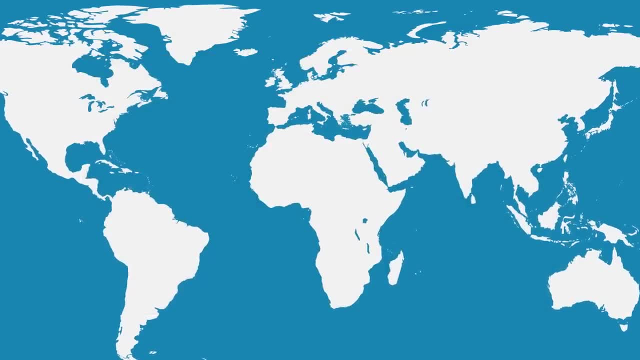 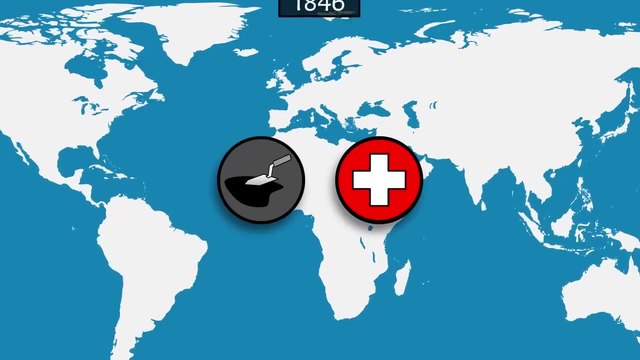 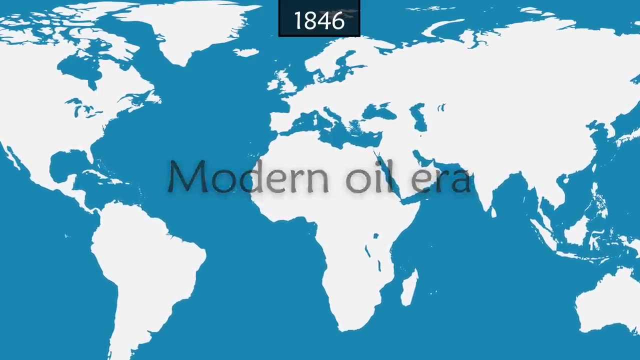 to man. since ancient times Around the world, oil was used as sealing material, in construction and for medical purposes, But it is only in the middle of the 19th century that its consumption would explode. Europe and North America, in the midst of industrial revolution, have rapidly increasing. 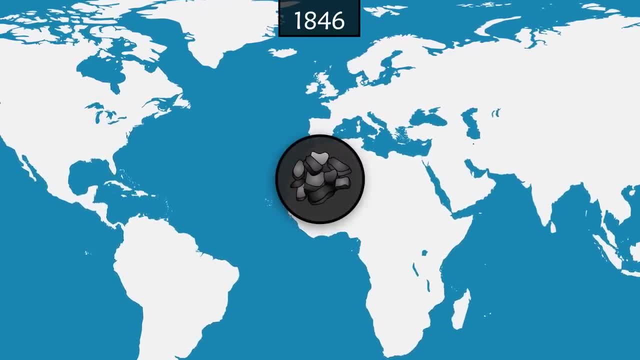 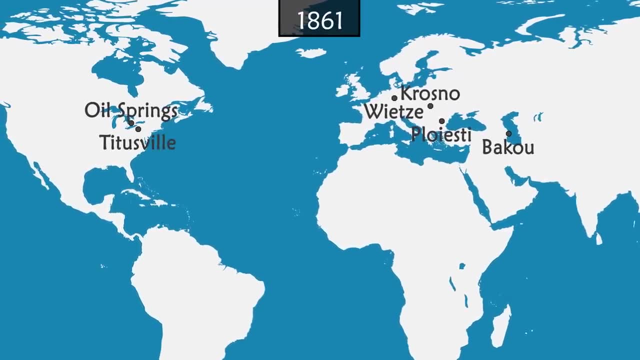 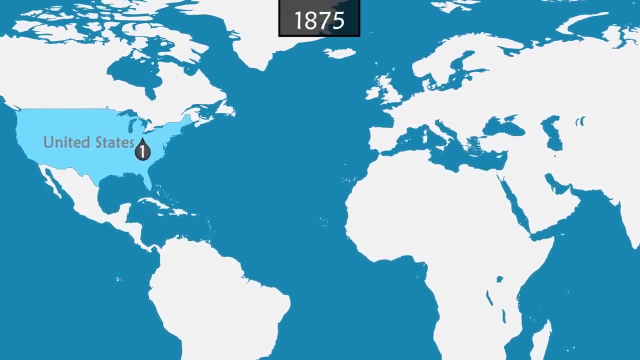 energy requirements that are met mainly by coal. Interest in oil intensifies throughout the world, from the Russian Empire to Europe, to North America. the first modern drilling location In the United States. this causes a rush of black gold and the country becomes the largest. 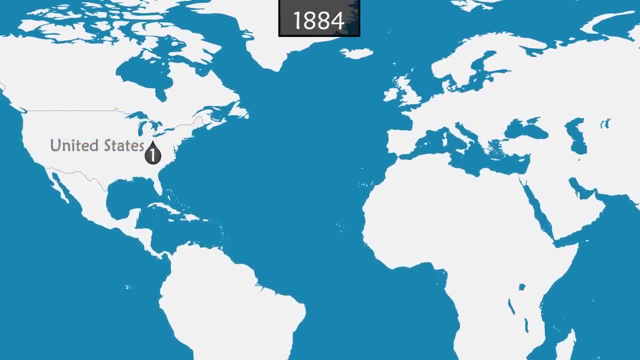 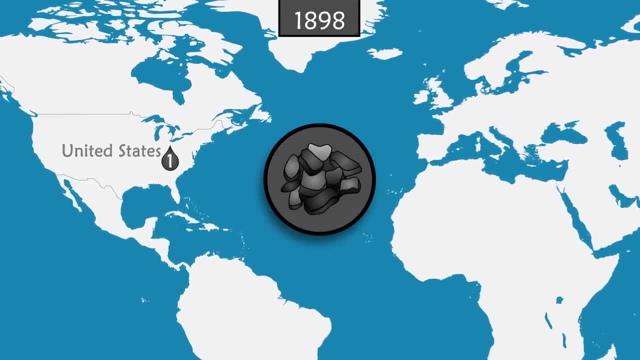 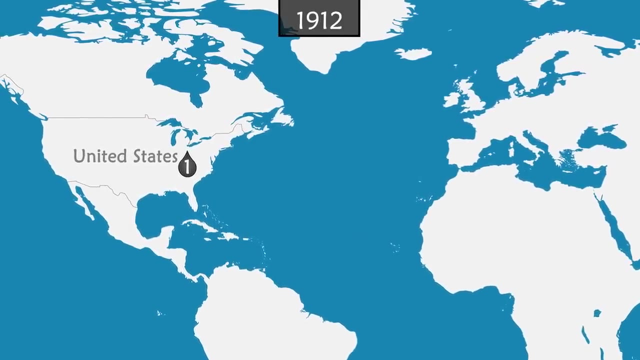 oil producer in the world. Initially distilled oil replaces the burning of whale oil in lamps. It offers a better calorific value than coal and is easier to transport than gas. Oil consumption rises in the early 20th century, especially in the field of transport, with the development of 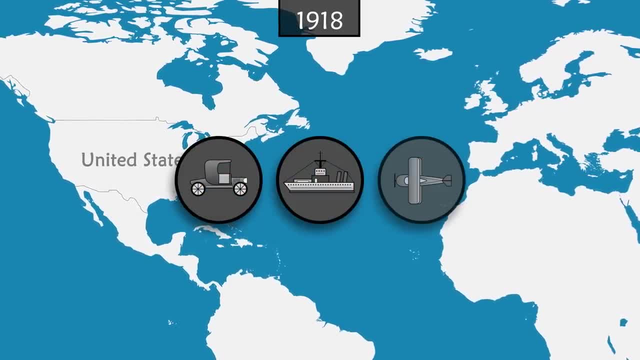 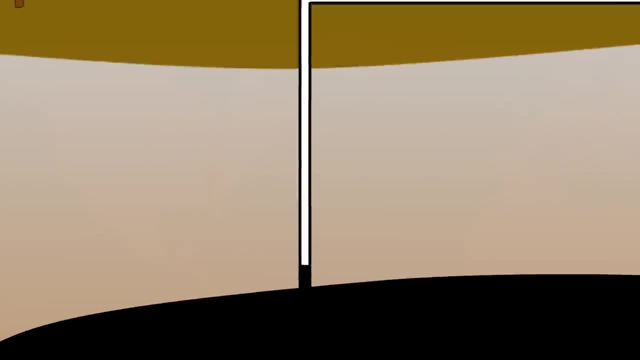 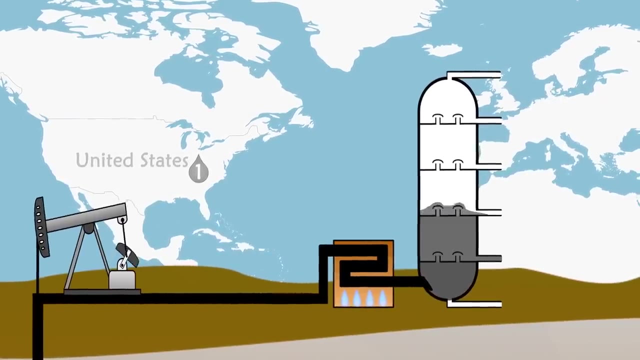 the automobile, the reconversion of ship engines and the aviation boom during World War I. Crude oil, once extracted, is distilled in a refinery to separate the hydrocarbons as needed. The lighter molecules evaporate to the top of the distillation column, where the temperature is around 20 degrees Celsius. Liquefied petroleum: 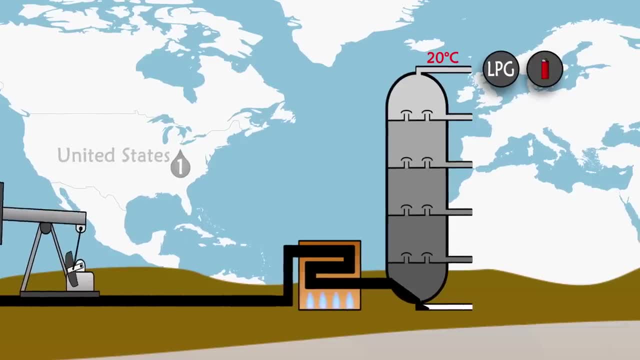 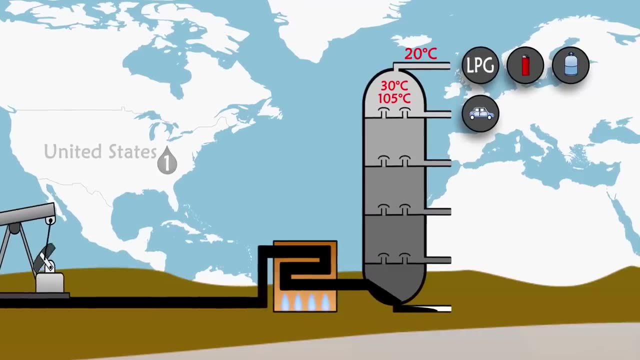 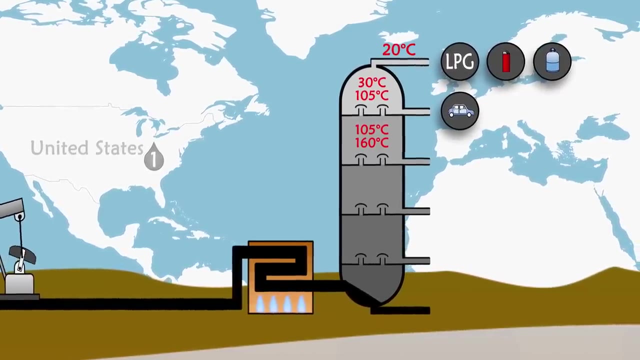 gases are harvested and used, among other things, in lighters and in kitchens Between 30 and 105 degrees Celsius. gasoline for cars is produced Between 105 and 160 degrees Celsius. naphtha is created, used in petrochemicals in order to create plastics, synthetic textiles, drugs. 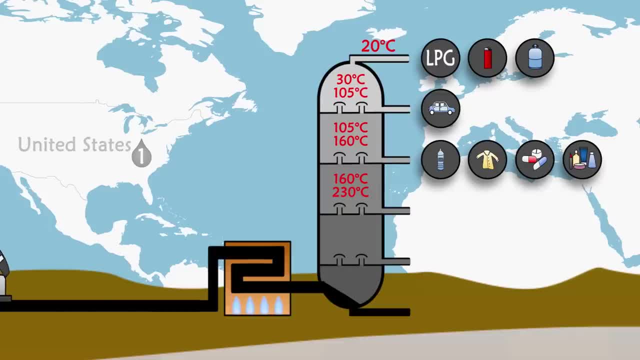 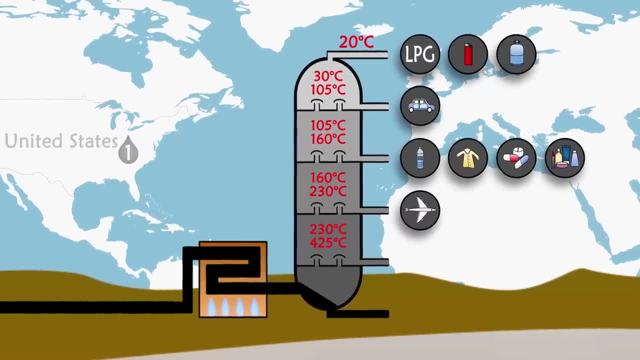 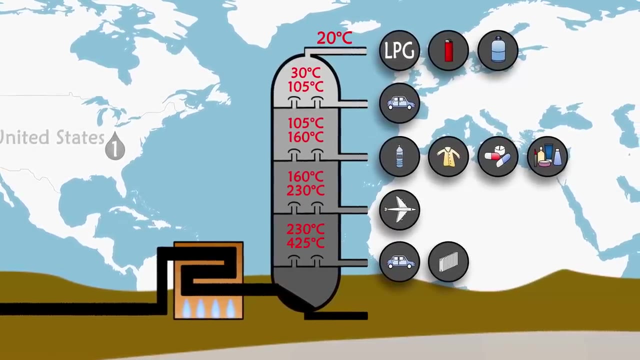 and cosmetics Between 160 and 230 degrees Celsius. kerosene is obtained for aviation Between 230 and 425 degrees Celsius. diesel is created for cars and heating oil for domestic purposes. Finally, the thick high-sulfur residue is heated to above 450 degrees Celsius to form. 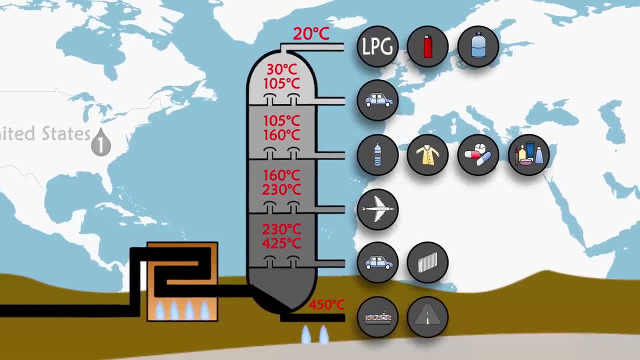 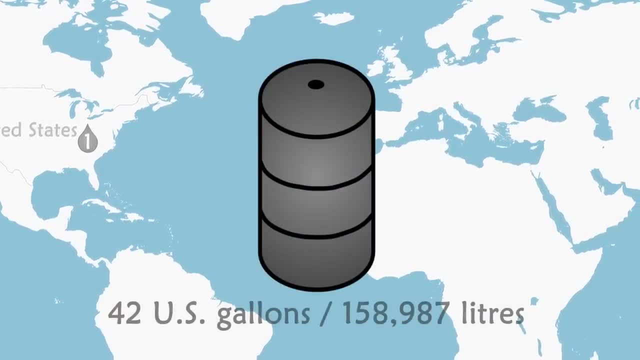 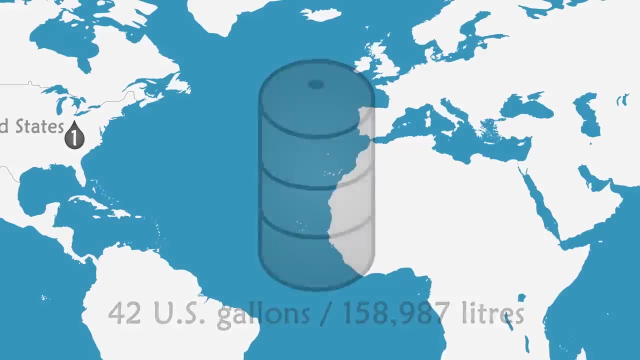 heavy fuel oil used by ships. This heavy fuel oil is used for road construction and roofing. Crude oil was transported in barrels with a capacity of 42 US gallons, or slightly less than 159 liters. The barrel thus became the unit for setting oil prices. 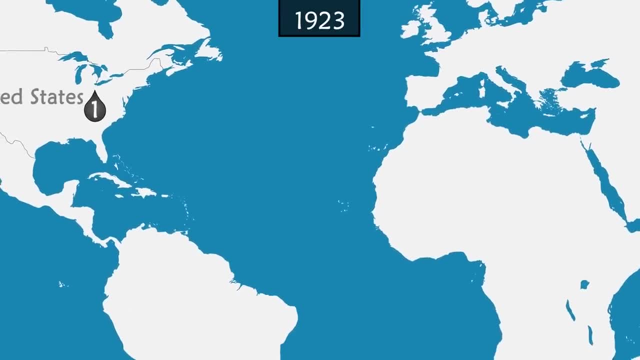 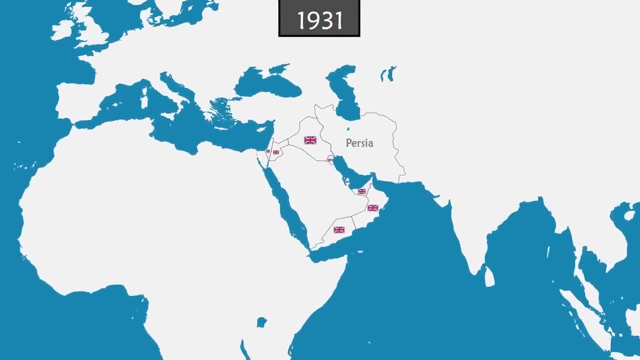 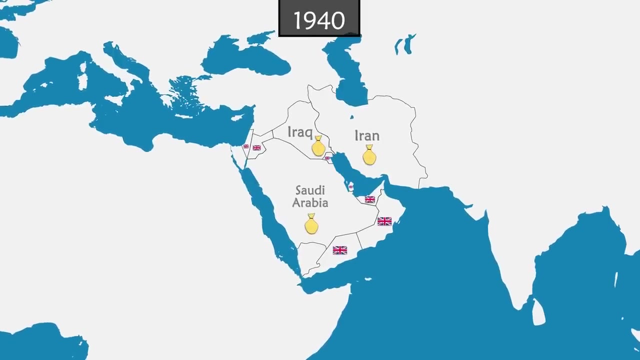 More and more oil deposit discoveries are made worldwide, including in Venezuela, which becomes the second-largest global producer. In the Middle East, where Britain is present, Western companies seize the new market, giving a portion of their profits to the local country through royalties. During World War II, demand for oil skyrockets and the resource becomes. 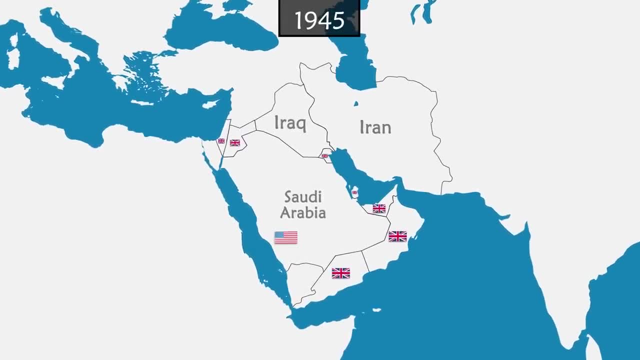 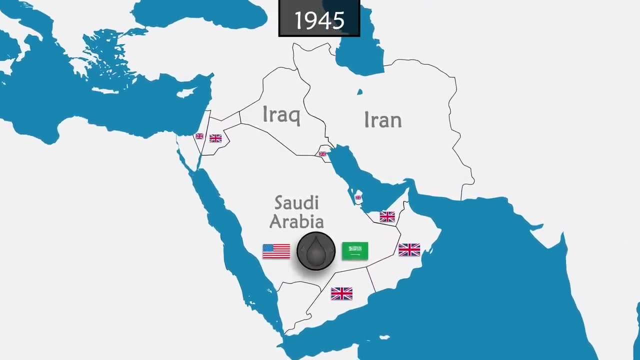 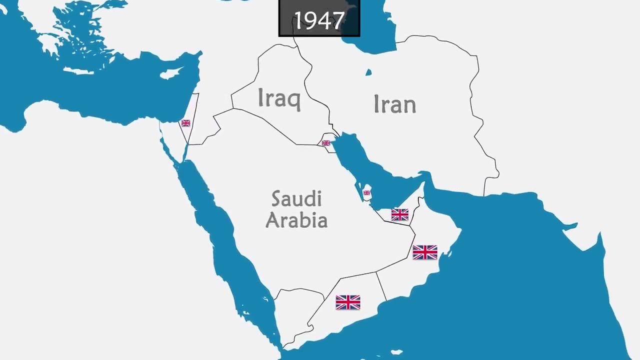 a major international issue. At the end of the war, the United States signs an alliance with Saudi Arabia guaranteeing security of the country in return for privileged access to its oil. Western companies dominating oil markets contribute to nationalist movements in producing countries. In Saudi Arabia, an agreement is signed allowing the country 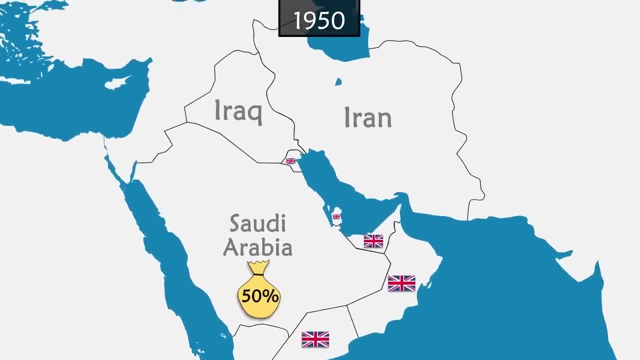 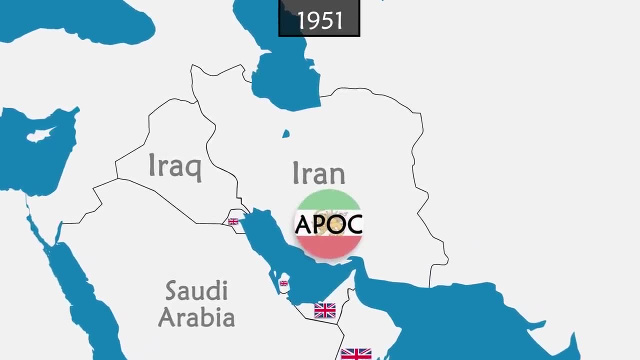 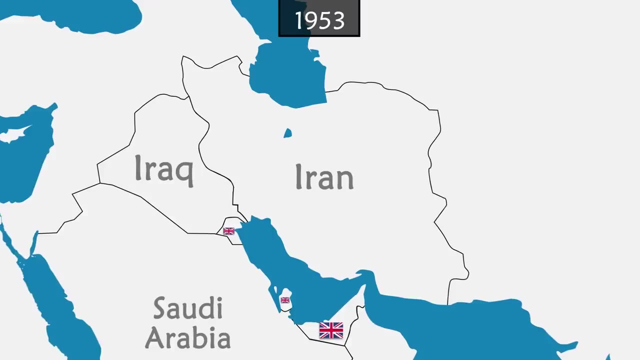 to receive 50% of oil profits In Iran. negotiations with the Anglo-Persian oil company fail, following which the Prime Minister nationalizes the country's oil. In response, the US and the UK secretly organize a coup to overthrow the Prime Minister. The Shah of Iran remains in. 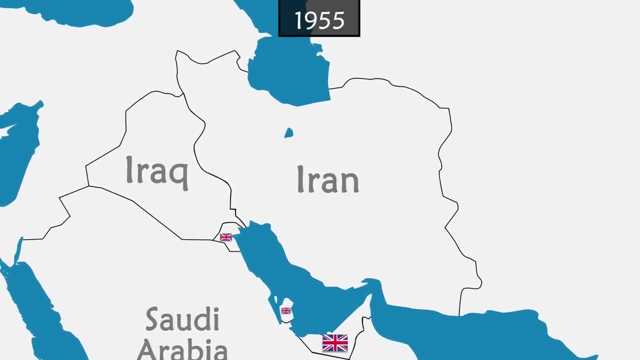 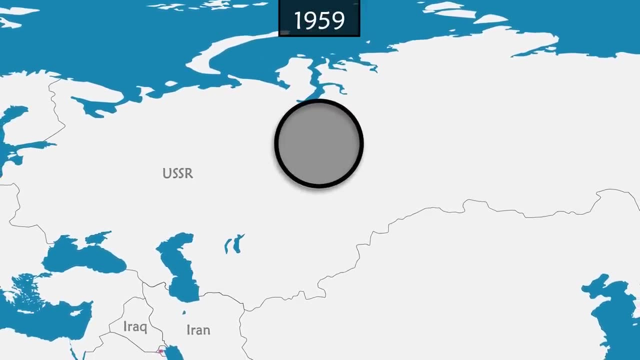 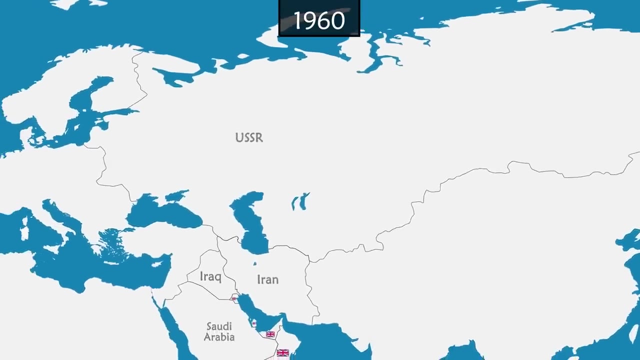 power and then allows the exploitation of oil in the country by a consortium of Western companies. In the USSR, the discovery of oil fields in Western Siberia pushes the country to invest in its exploitation. Plentiful and cheap oil overtakes coal to become the primary source of energy in the 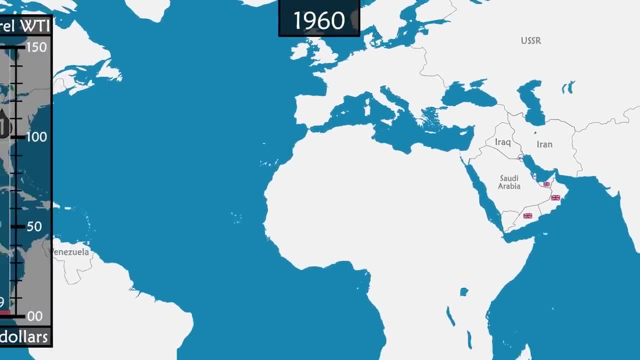 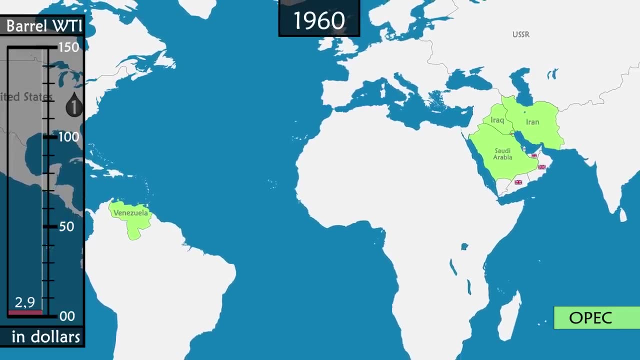 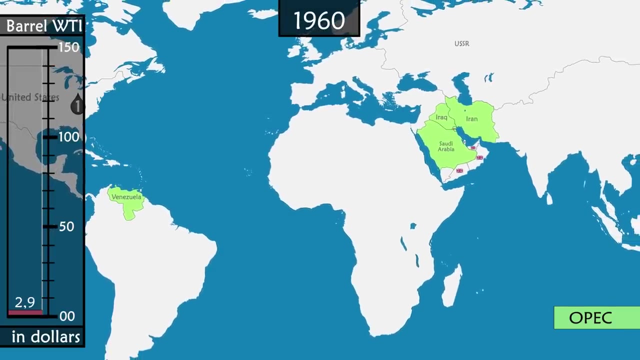 world. So far its price remains below $3 a barrel. Five major oil-producing countries decide to unite to derive more benefits. They create OPEC, the Organization of Petroleum Exporting Countries, But together they want to counter the dominance of Western companies to increase oil prices. 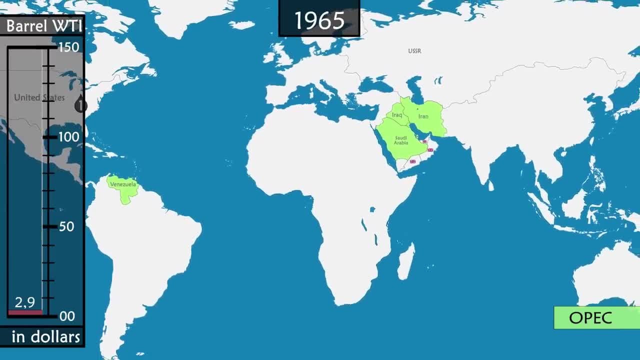 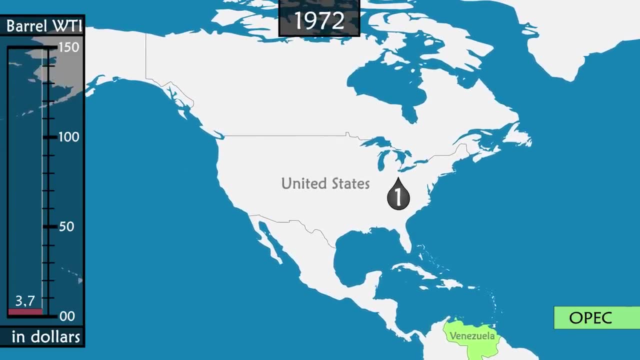 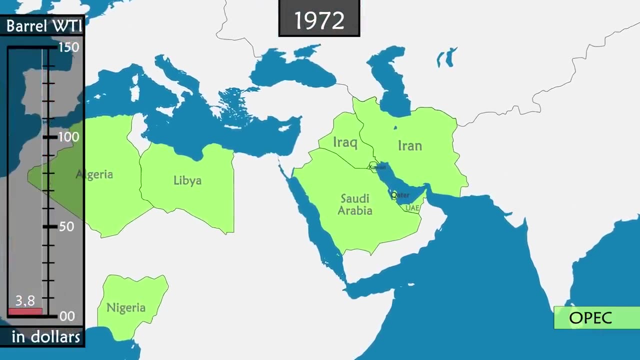 and to have a common policy. The organization would gradually be joined by new nations. In 1972, the United States reaches peak production and is forced to import oil to meet its increasing needs. As the United Kingdom withdraws from the Middle East, security in the region is. 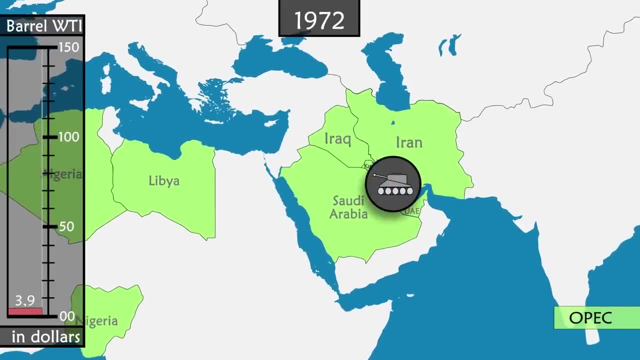 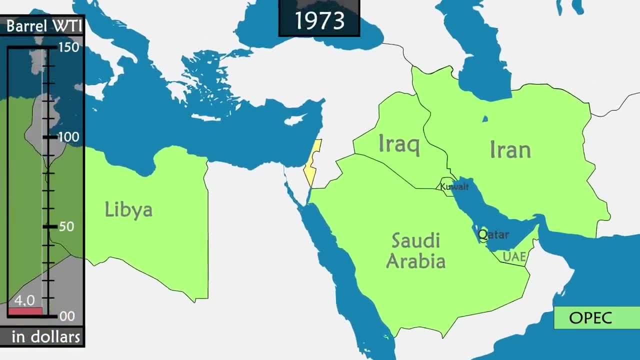 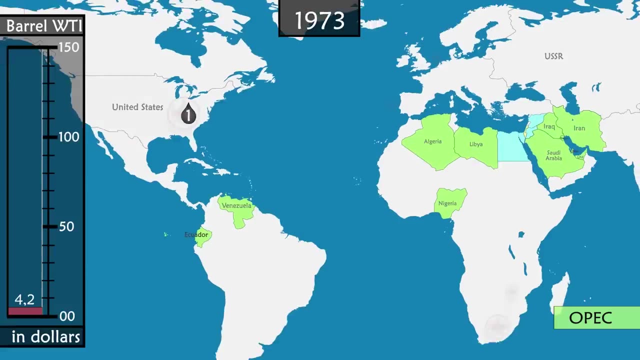 provided by Iran and Saudi Arabia, which are armed by the West. After the Yom Kippur War between Israel and the Arab states of Egypt, Syria and Jordan, OPEC for the first time uses oil as a political weapon. An oil embargo is imposed on Israel's 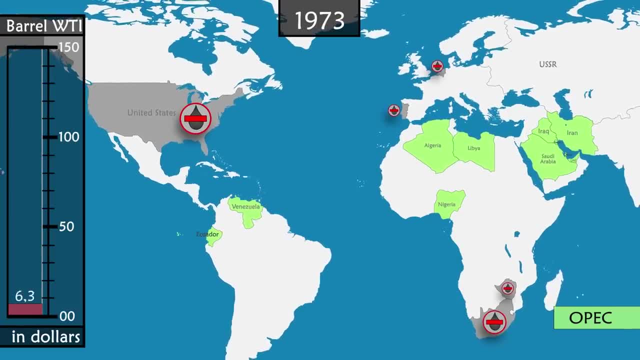 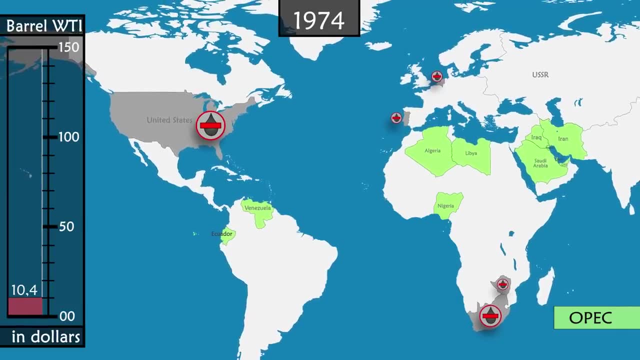 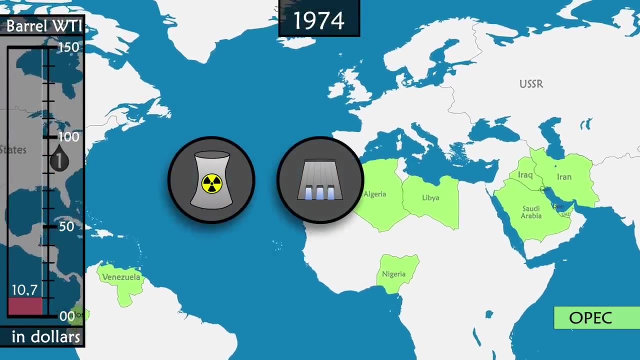 allies and production slows to inflate the price of oil. This is the first oil crisis which hits industrialized countries whose economies now depend on the black gold. Countries try to reduce their oil consumption and invest in alternatives such as nuclear and hydropower, or reinvest in coal. Oil companies in turn explore the world in search of new deposits. 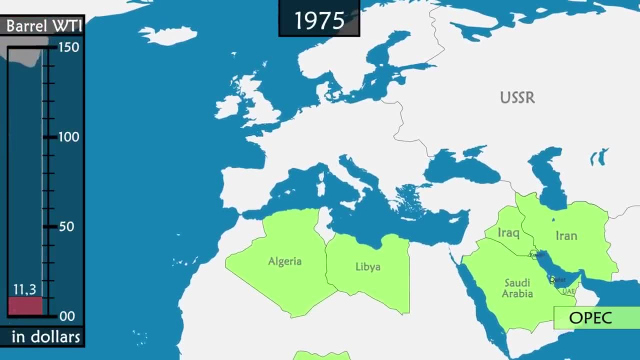 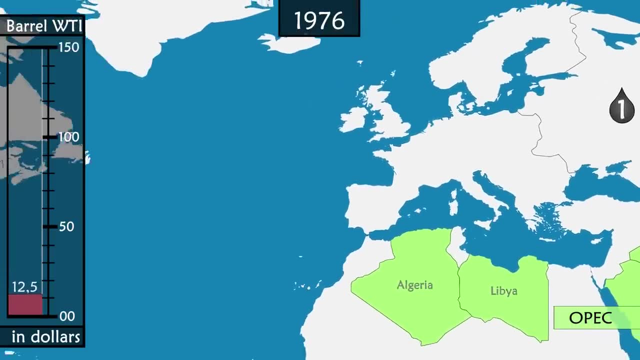 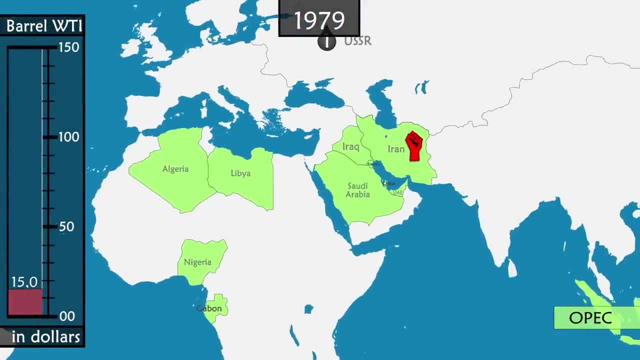 Sources at sea, called offshore sites, are discovered and exploited, particularly in the North Sea. The Soviet Union becomes the largest producer of oil in the world, while in the United States production increases with the exploitation of Alaskan oil. In 1979, the Iranian Revolution takes place. The Shah's regime is overthrown and replaced. 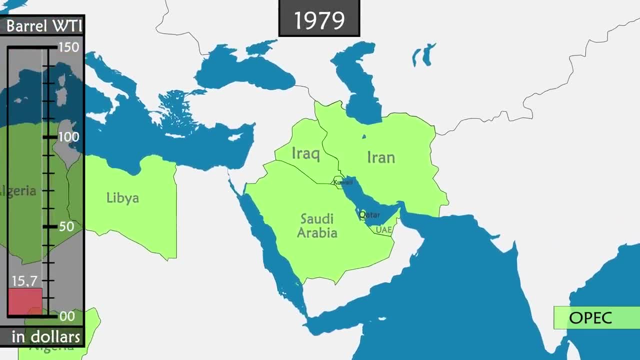 by an Islamic Republic. In 1979,, the Iranian Revolution takes place. The Shah's regime is overthrown and replaced by an Islamic Republic. In 1979,, the Iranian Revolution takes place. The Shah's regime is overthrown and replaced by an Islamic Republic. 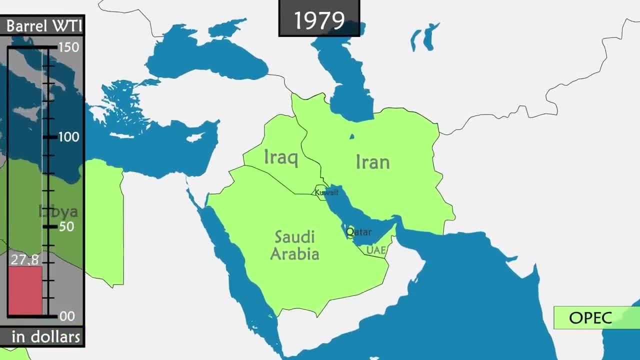 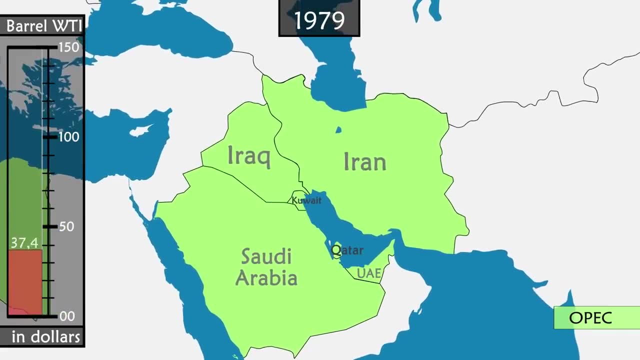 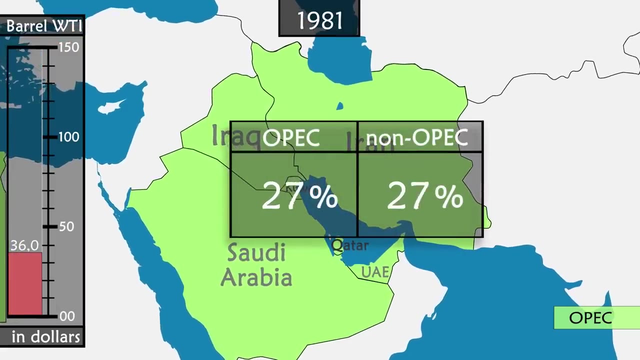 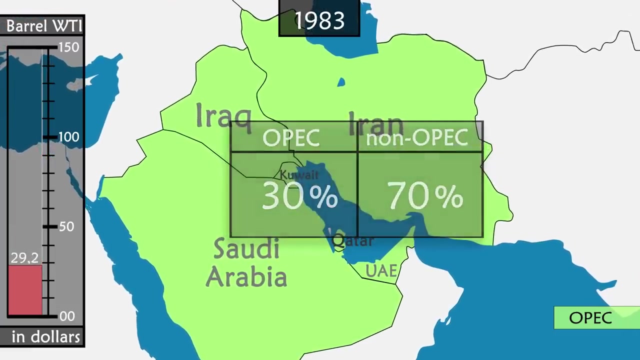 Oil production in the country falls, causing the second oil crisis Following border disputes. tensions between Iran and Iraq lead to eight years of war. Globally, non-OPEC oil production rises and exceeds production by OPEC countries. Henceforth, supply and demand sets the price for a barrel rather than OPEC. 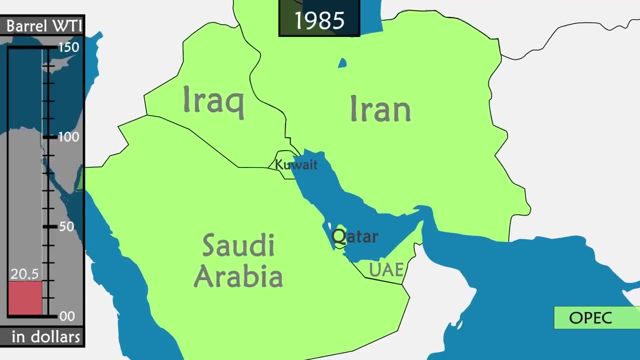 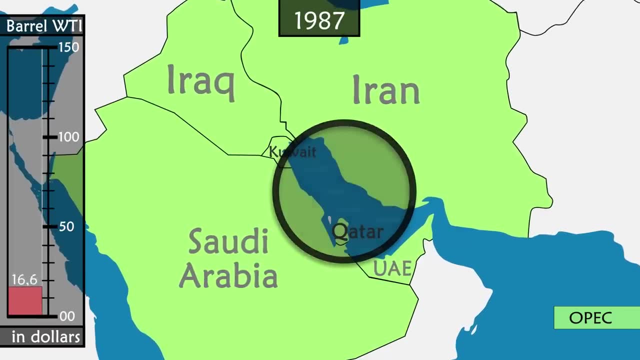 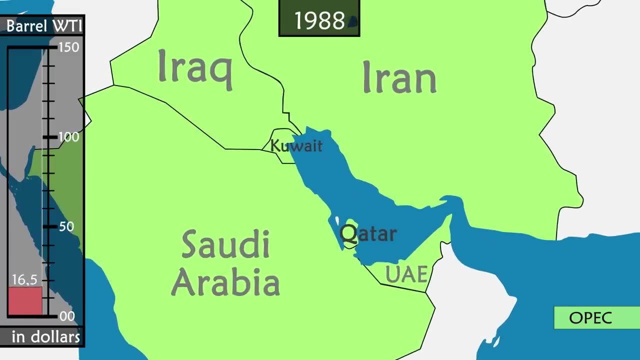 For industrialized countries, the stability of the Middle East still remains a priority. Thus, when Iraq and Iran begin to target oil facilities in the Persian Gulf, hundreds of Western military vessels step in to ensure the supply of oil. At the end of the war, Iraq is weakened and indebted to Saudi Arabia and Kuwait. But having 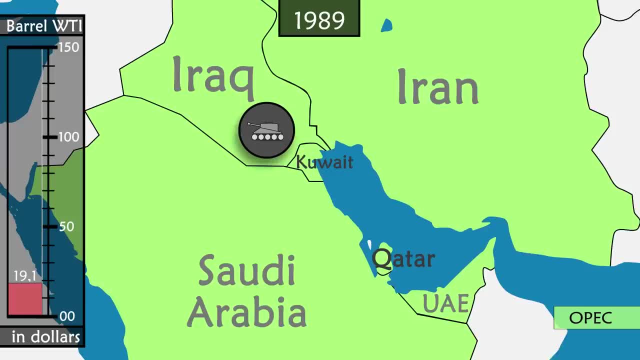 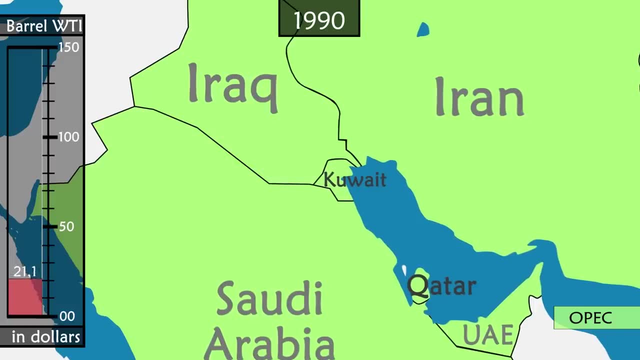 received large amounts of military equipment. the country has the most powerful army in the region. Iraq takes advantage of this situation to invade Kuwait with its military equipment. Iraq takes advantage of the situation to invade Kuwait with its military equipment. Iraq takes advantage of the situation to invade Kuwait with its military equipment. 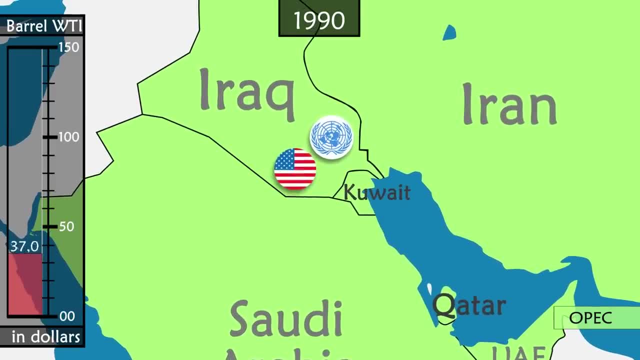 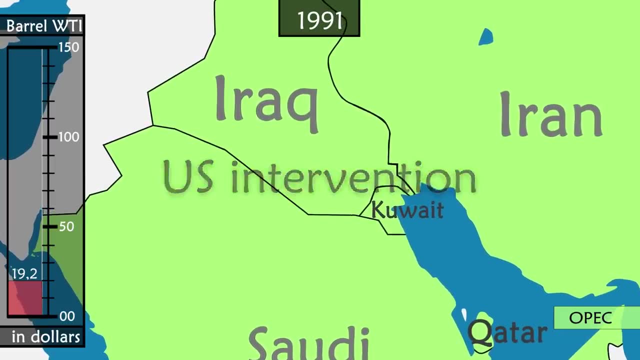 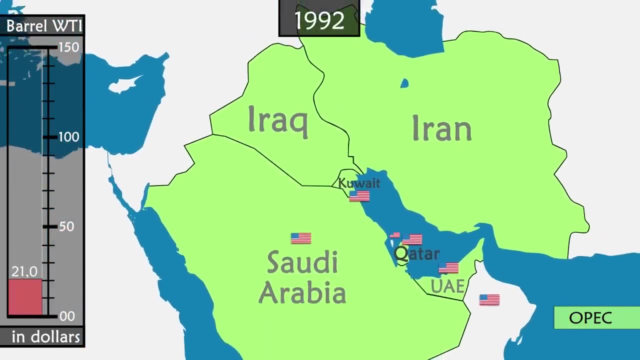 An international coalition is formed under the UN and led by the United States to intervene and neutralize the Iraqi Army. This time, the United States establishes a permanent presence in the region by installing military bases and signing defence agreements with Gulf monarchies. These current riots come as believing a terrorist threat comes a typhoon. 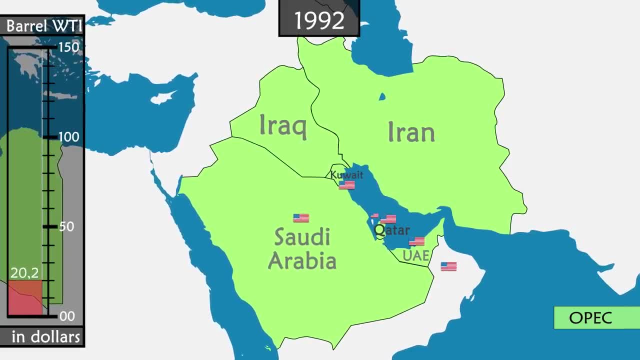 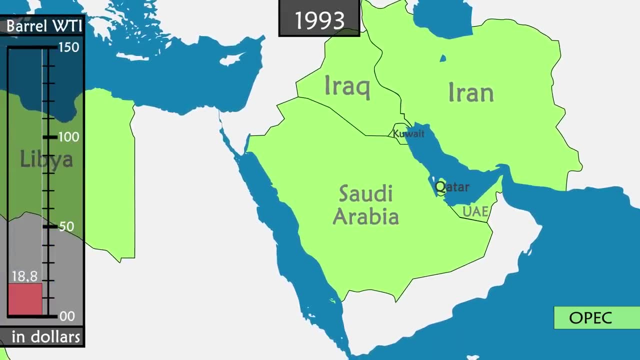 Iraq forever will see an increasingly sabotage campaign. the Ev首先 hits the пред Islander from the Gulf toatar and its panther army. The State disposes a series of hahk hey kosher ins slots against Iran and Ira k k. its part, wants to once again become a major producer of oil. 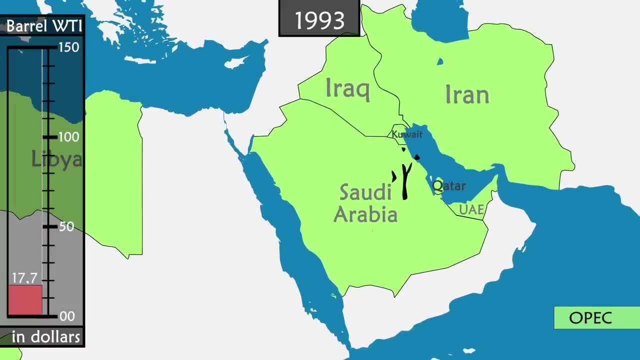 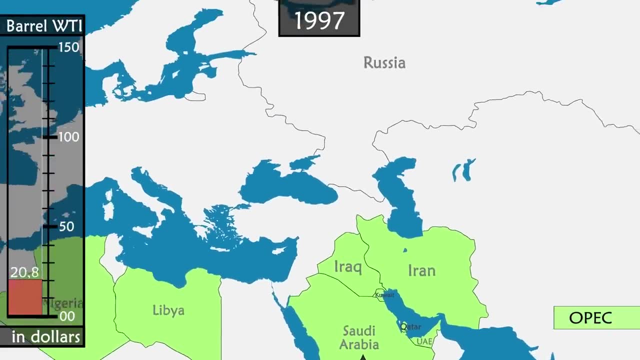 The country has the largest known oil reserves in the world and floods the market to become the largest producer of crude In Russia. new investment revives the oil industry, But as the price of oil is low and offshore operations unprofitable, oil companies find. 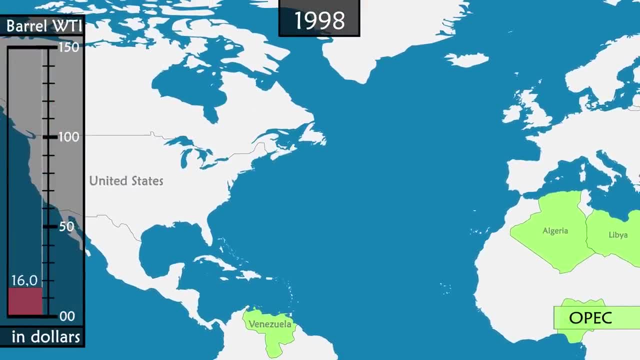 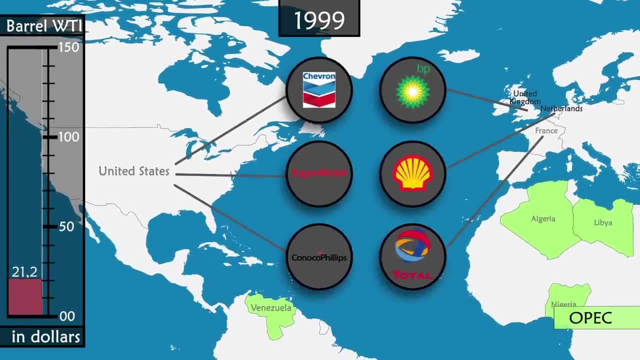 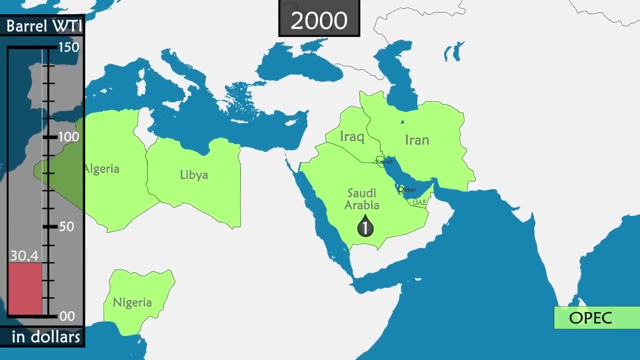 themselves in difficulty. In 1998, they begin to merge together and combine forces. Six giant oil companies are born that would become the richest and most influential in the world. In the Middle East, the military presence of the United States begins to raise concern. 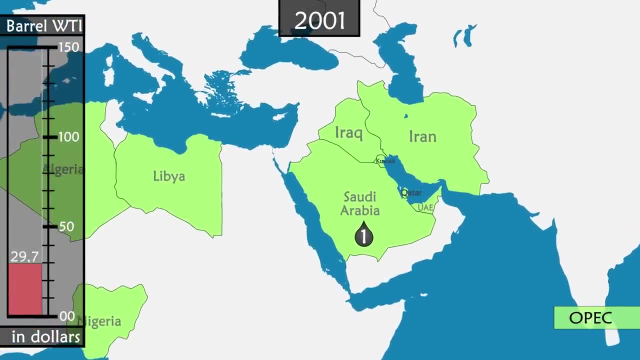 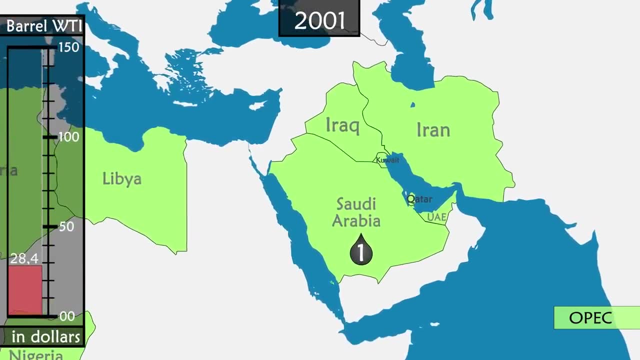 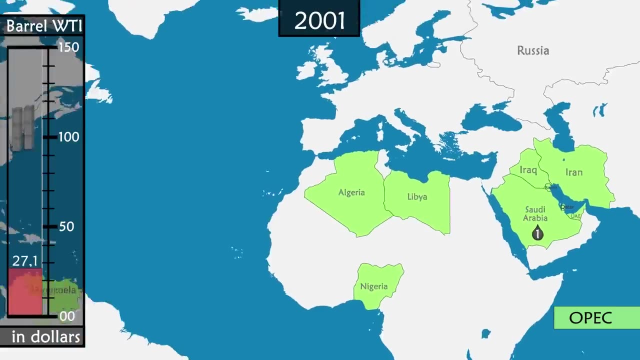 On one hand, radical Islamists do not want the presence of an Israeli ally on their soil. On the other, some consider the sanctions imposed on Iraq and Iran as too heavy. On September 11, 2001,, the United States becomes the top oil company in the world. 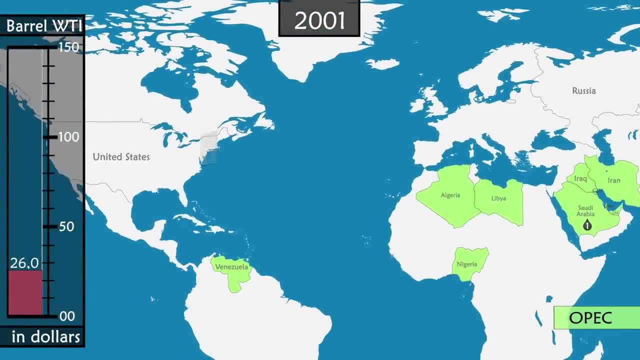 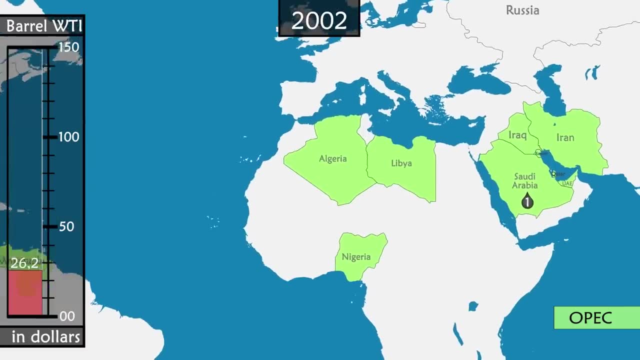 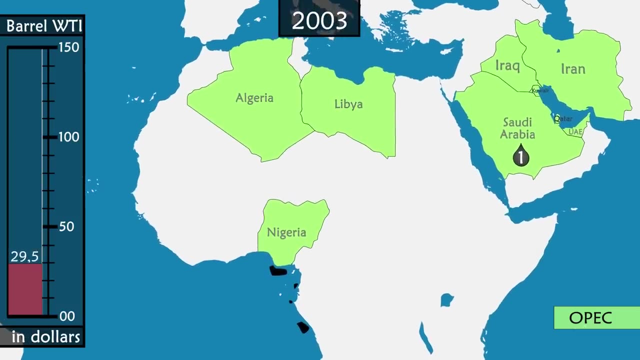 Iraq is the target of a major terrorist attack on its territory. Fifteen of the nineteen terrorists were Saudis, raising grave concerns. The US actively seeks new sources to reduce oil dependency on the Saudis. In Africa, production accelerates after the discovery of large offshore fields off the 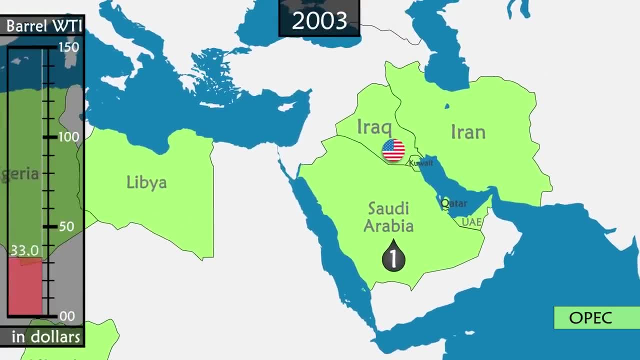 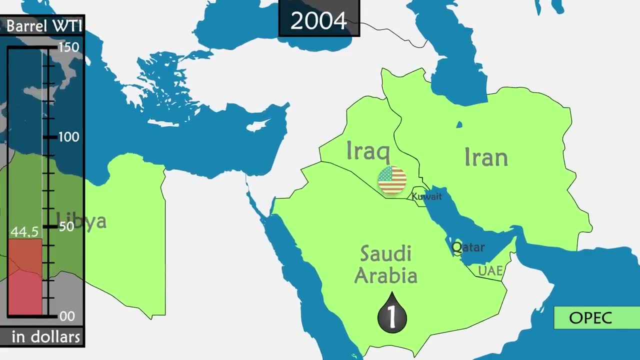 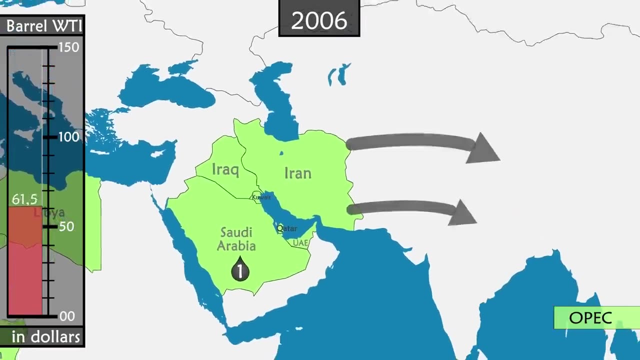 Gulf of Guinea. In the Middle East, the United States invades Iraq under the pretext of its war against weapons of mass destruction. A few years later, the country's oil would be back on the ground. Iran, for its part, opens its market to new rising Asian powers, such as China and India. 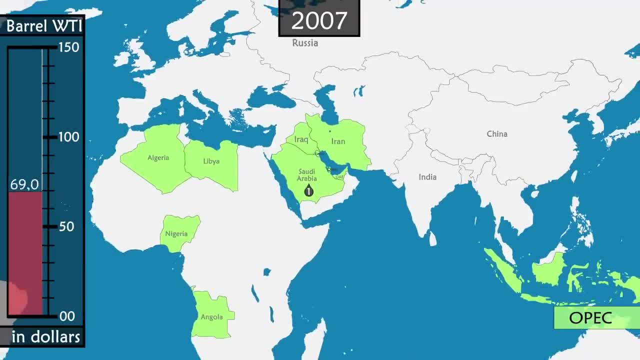 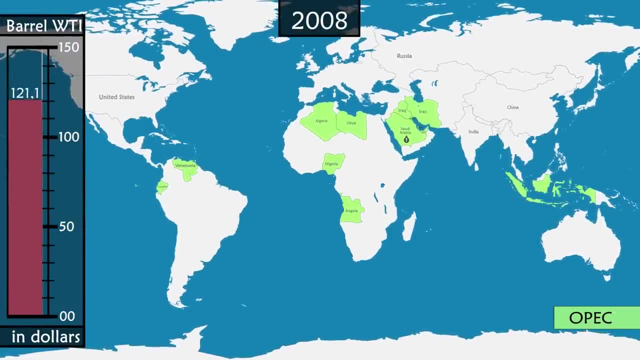 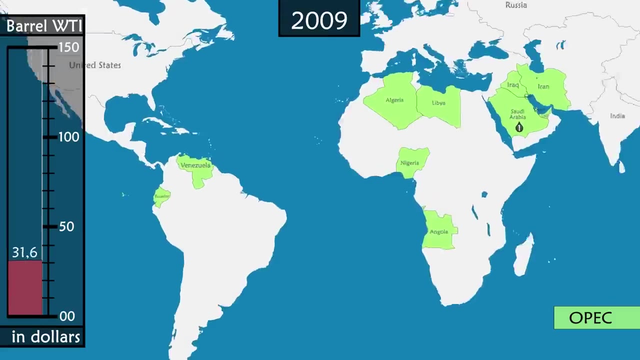 The abundant supply of oil in the world stimulates the economy. Growth skyrockets, mainly in emerging countries. In addition, Wall Street traders speculating on black gold push prices further upward, But the financial crisis of 2008 would cause a sharp drop in prices. 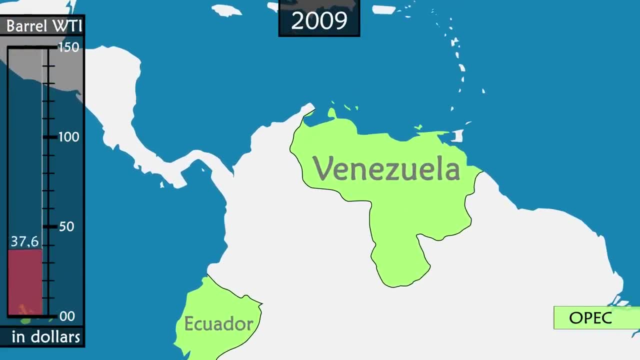 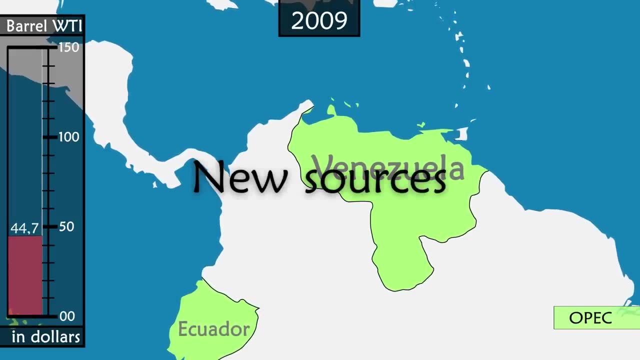 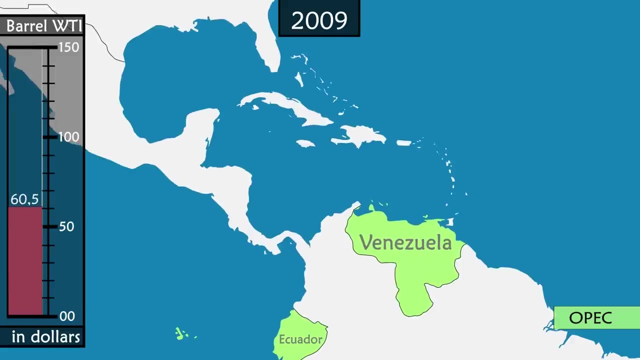 Venezuela, over a few years, discovers it holds the largest known oil company in the world, putting it ahead of Saudi Arabia. With more global demand for oil, its price rises again. The unconventional exploitation of petroleum becomes profitable, despite the difficulty in its pumping and treatment. 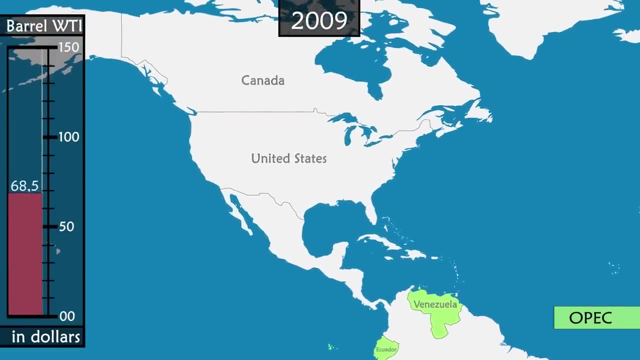 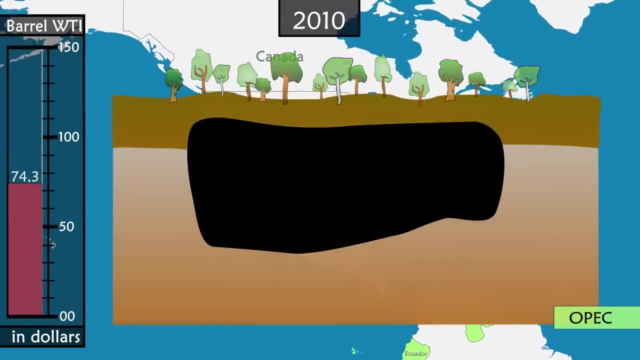 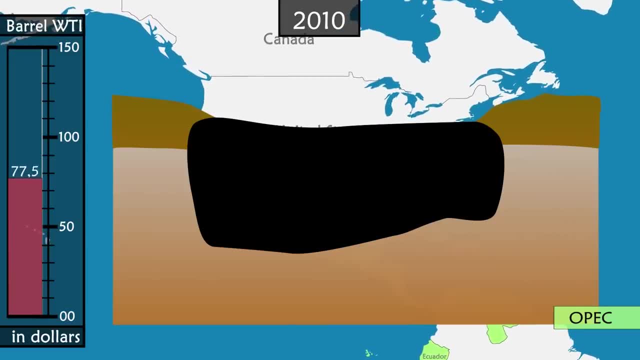 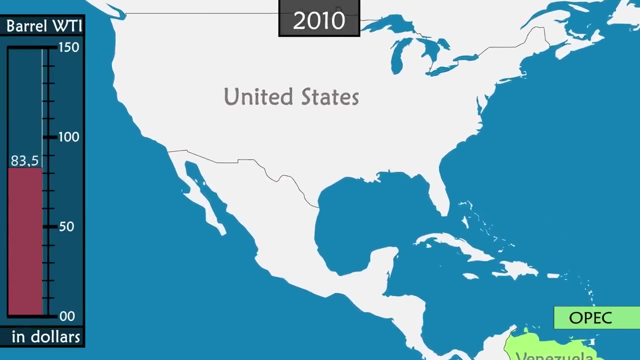 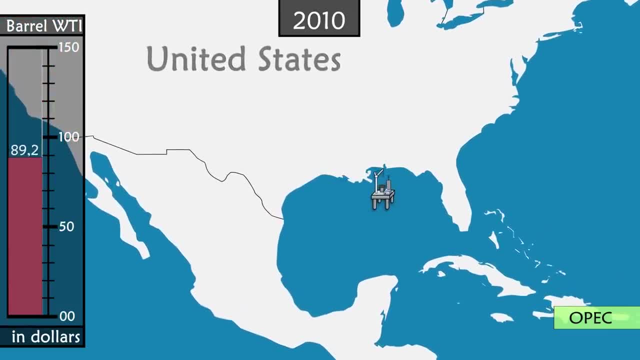 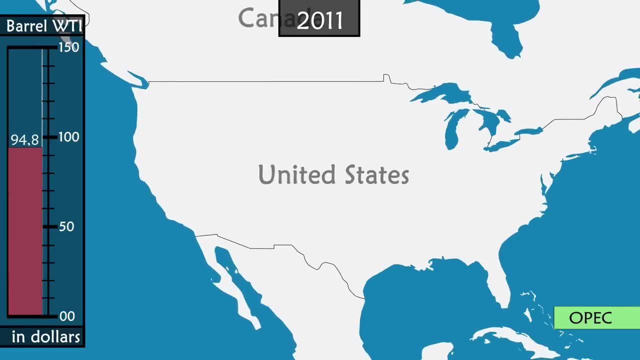 ens to extract from the oil. It is then transformed with more expensive, highly polluting techniques. While Offshore now provides 30 percent of global production, oil companies try exploiting deeper deposits In the Gulf of Mexico. an attempt to make the deepest borehole in the world fails, causing 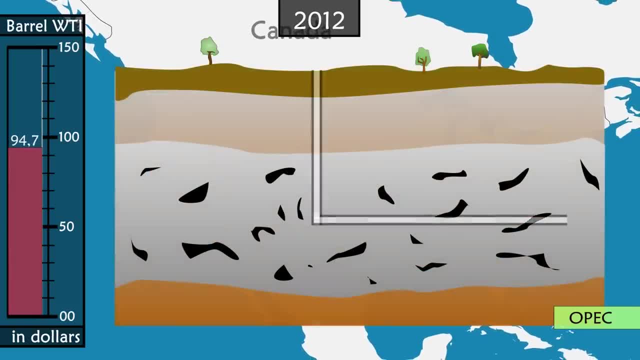 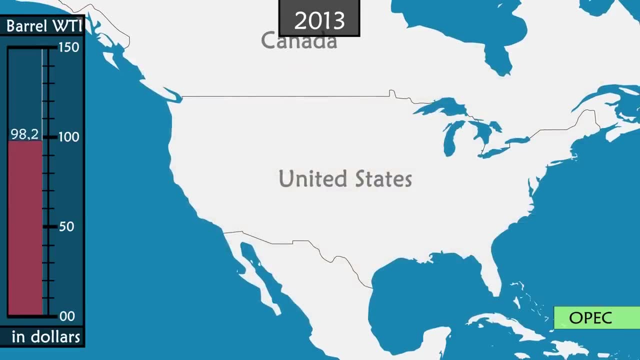 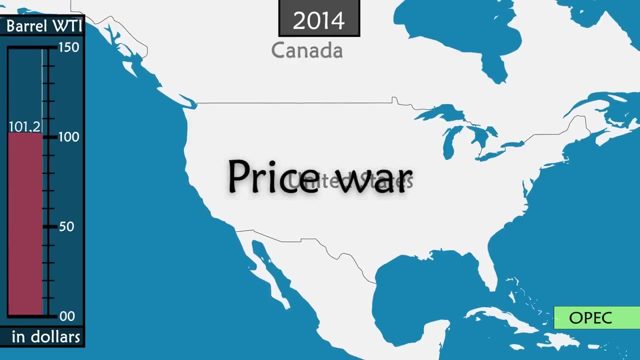 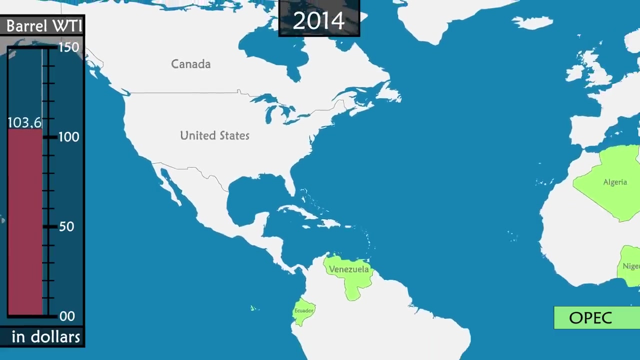 This oil is wedged between different layers of solid rock. A fluid is injected at high pressure to break the rock and release the black gold which is then pumped. Numerous such reserves discovered in the United States cause the country's production to explode. The fact that the biggest oil consumer in the world becomes a bigger producer does not please its Saudi ally. 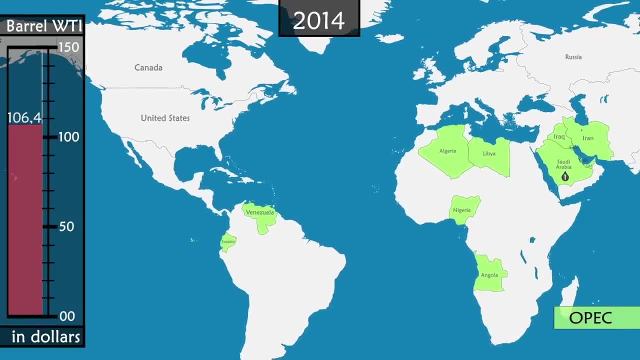 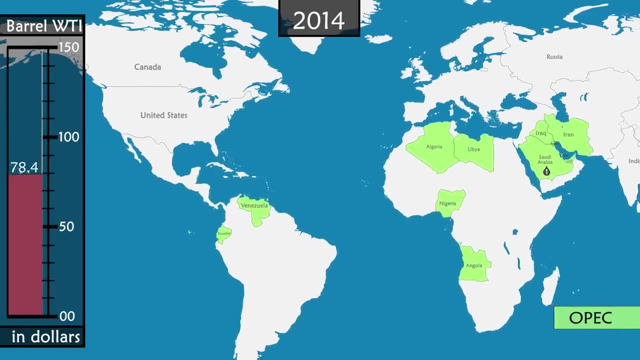 Saudi Arabia then wants to make the production of unconventional oil unprofitable by dropping prices. To achieve this, Saudi Arabia persuades OPEC to flood the oil market. The price of the barrel drops, making oil production barely, or sometimes not at all, profitable. 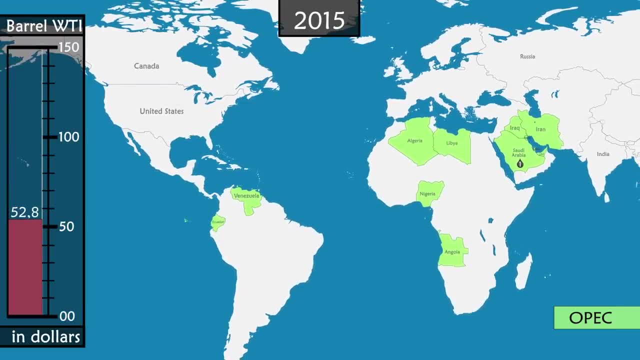 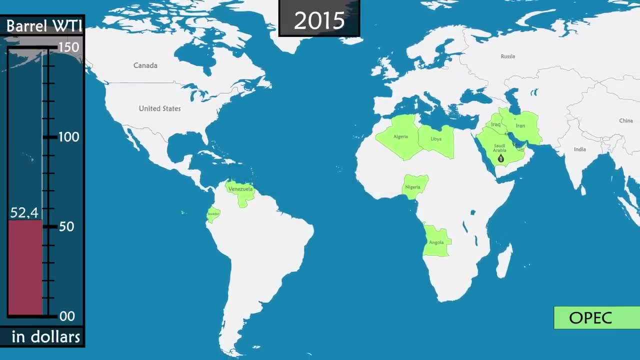 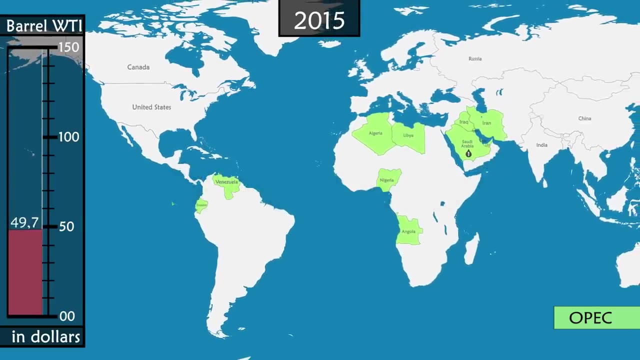 But the oil industry of the United States resists and continues to increase its production. With oil abundant and cheap, world consumption continues to rise and approaches 100 million barrels per day. Two-thirds of the oil used in the transportation industry is the main emitter of carbon dioxide. 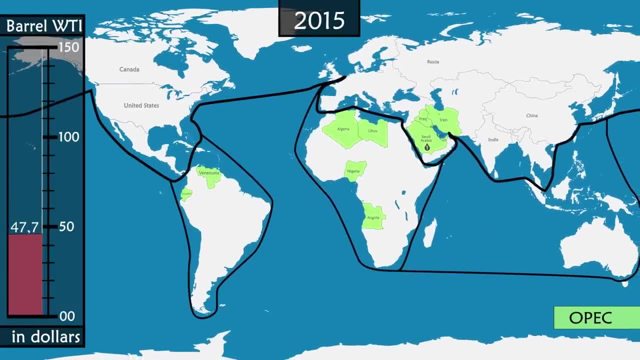 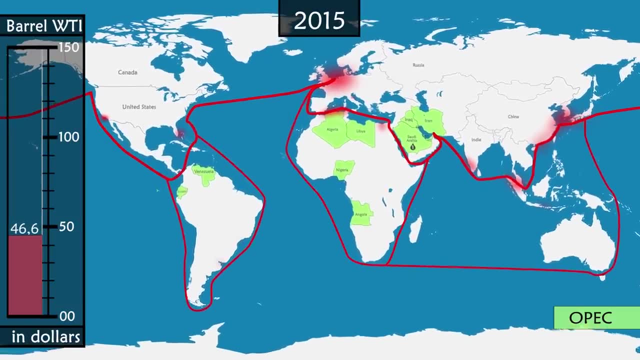 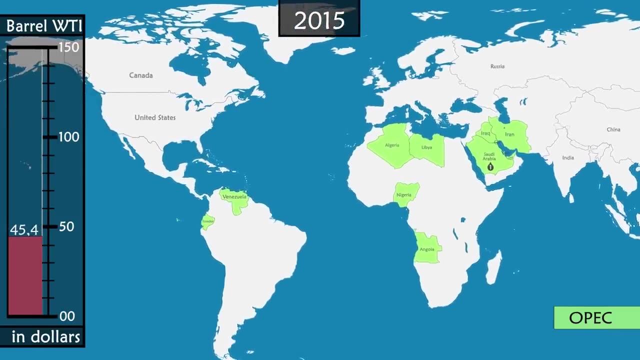 In the maritime sector. heavy fuel oil used by ships emits 3,500 times more sulfur than diesel fuel, causing severe air pollution. The United States and Europe react by creating zones where heavy fuel consumption is prohibited Since the beginning of the modern era of oil. 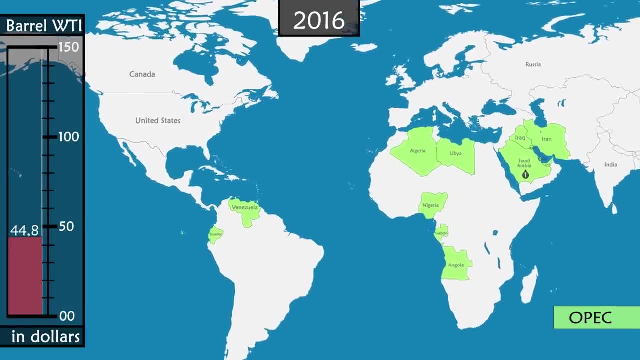 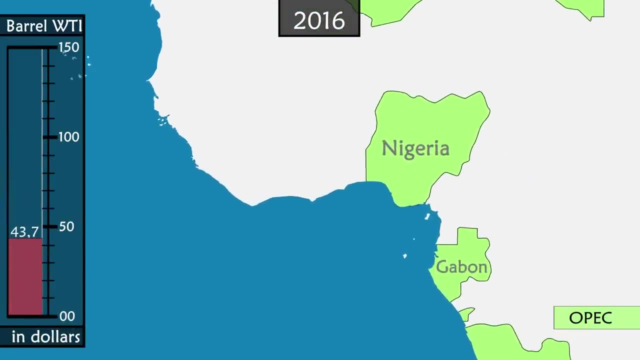 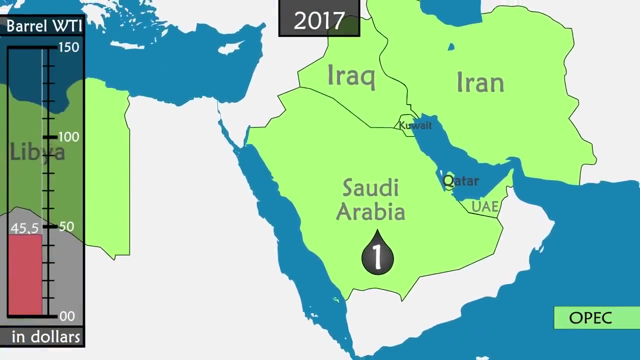 many oil companies have stopped producing oil. Oil spills cause major environmental damage, with the Niger Delta probably being the most affected region, with 60 years of oil spills. largely ignored, Saudi Arabia undergoes its own policy changes, being faced in recent years with a large fiscal deficit. 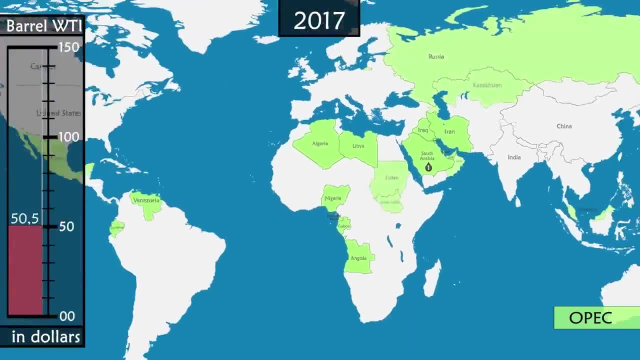 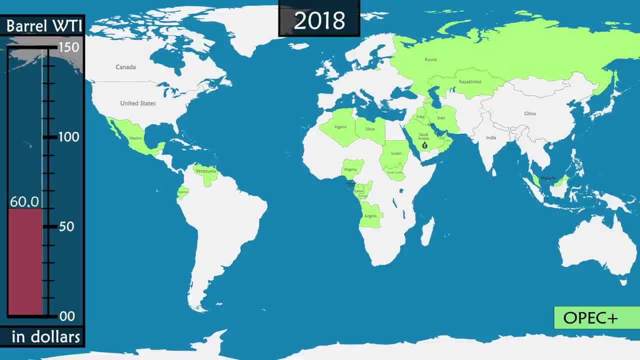 OPEC countries are forced to appeal to other producing countries to together try boosting the price of oil. This includes Russia, which is the world's largest crude exporter in the world. The United States, in contrast, continues to increase production to keep prices low. 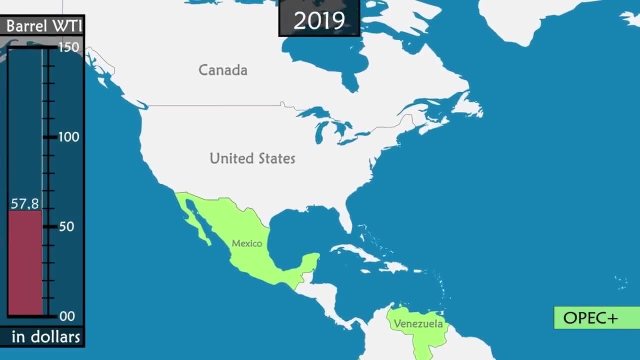 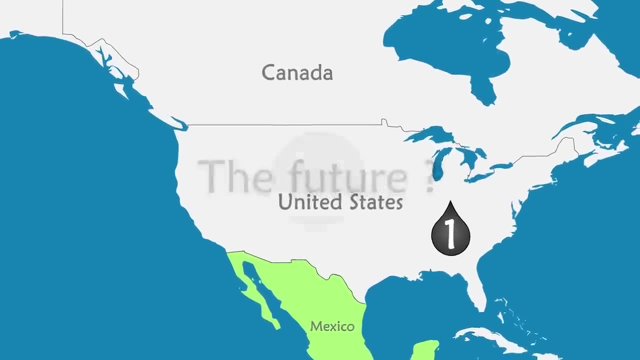 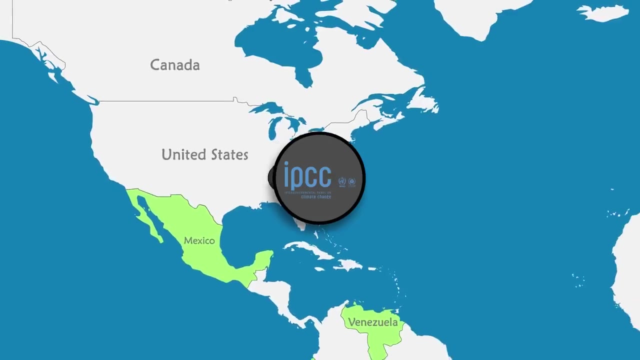 and to support growth and the economy. The country eventually becomes the largest oil producer in the world. While IPCC experts are sounding the alarm and call for drastically reducing CO2 emissions to limit global warming, we have currently found enough oil to carry on for at least another 50 years at current rates. 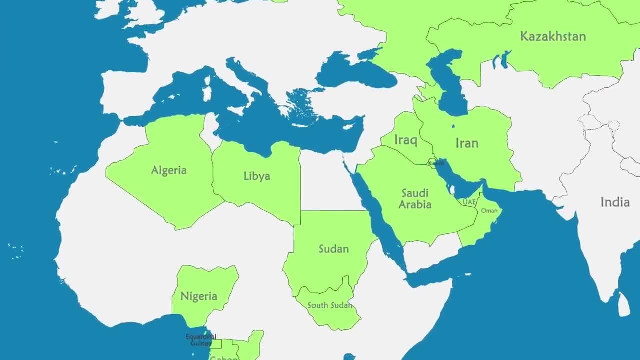 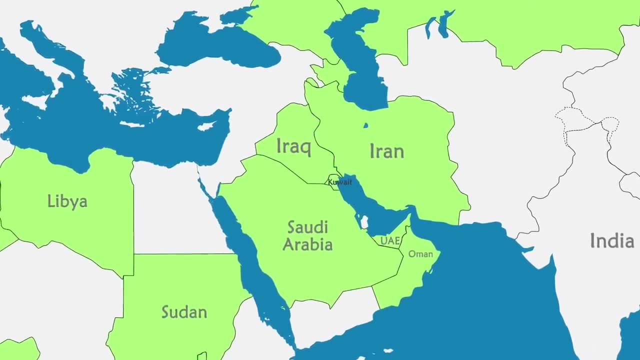 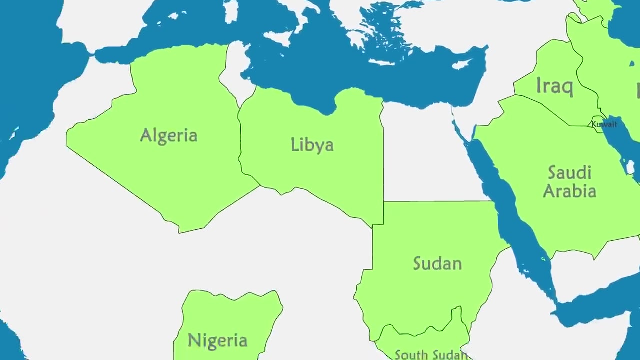 Saudi Arabia now speaks of diversifying its investments to prepare for the post-oil era. Iran, which has the third-largest oil reserves in the world, suffers since 2018 from sanctions imposed by the United States aimed at choking its oil sales. In Venezuela, the country is hurt by low oil prices. 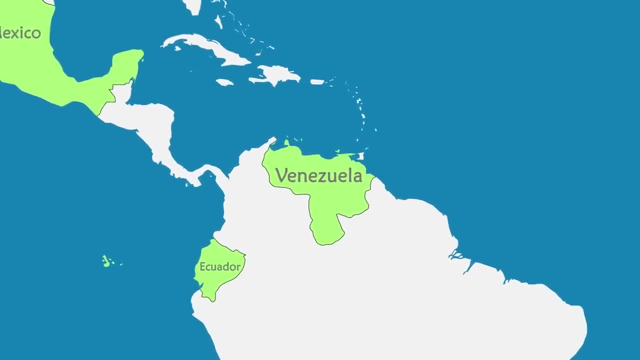 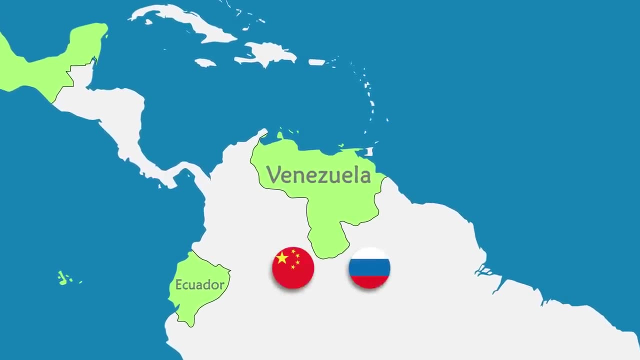 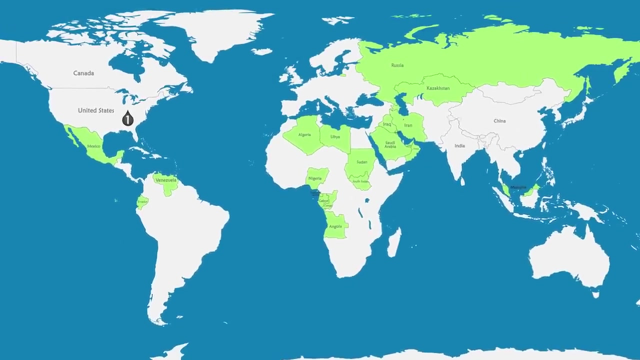 and the country never really benefits from its huge reserves. Political instability could potentially impact exports, which currently mainly benefits China and Russia. Meanwhile, oil companies remain among the most powerful entities in the world In 2017, five of them figure in a list of global top 10 companies. 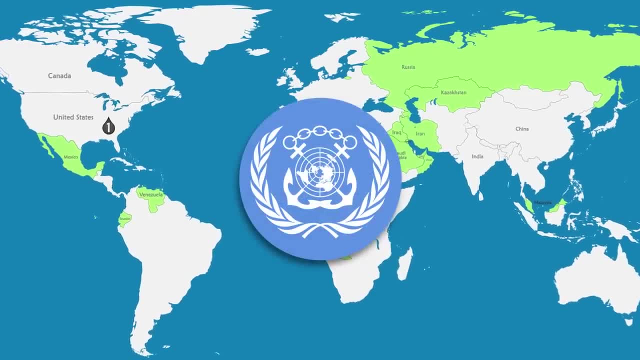 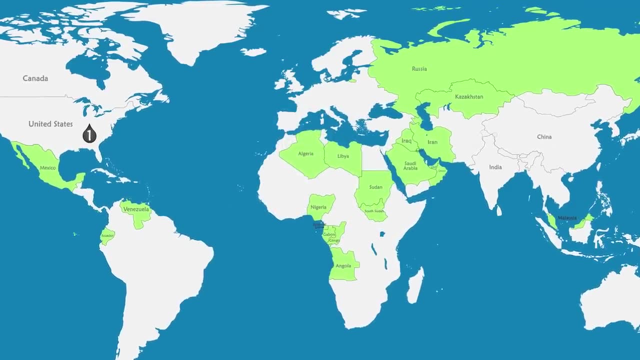 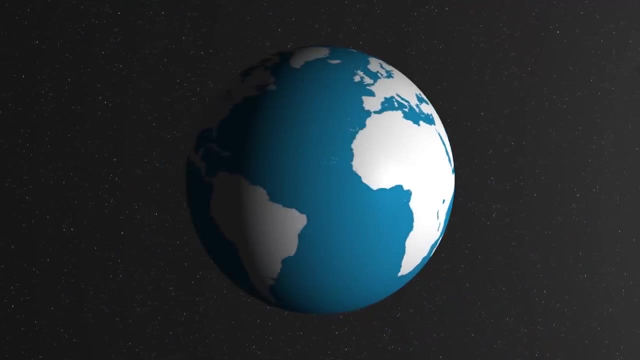 with the highest turnover. The International Maritime Organization imposes drastically reduced sulfur emissions goals for vessels by 2020.. This could force the industry to abandon heavy fuel oil in favor of other hydrocarbons, which may push up its demand and price If the price of a barrel increases. 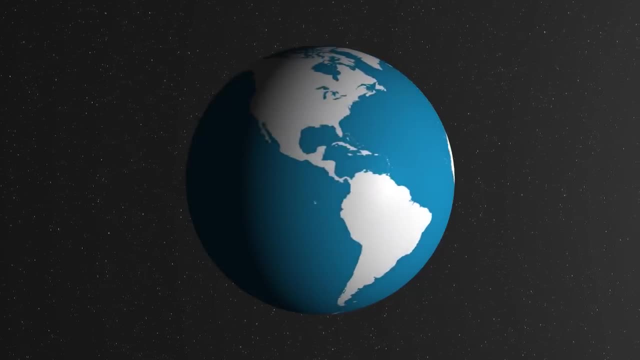 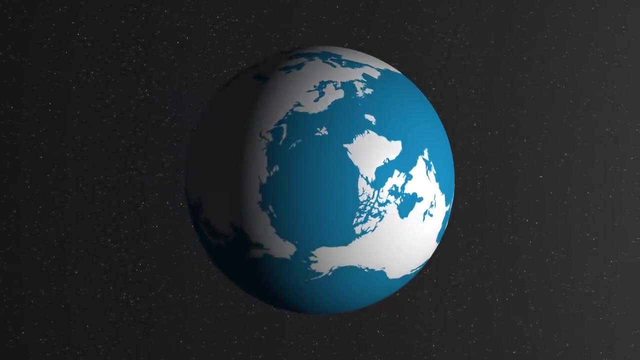 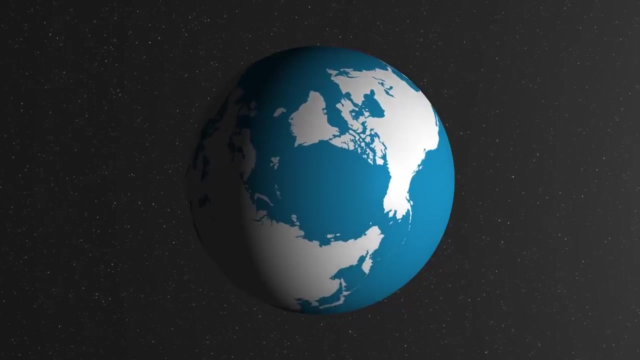 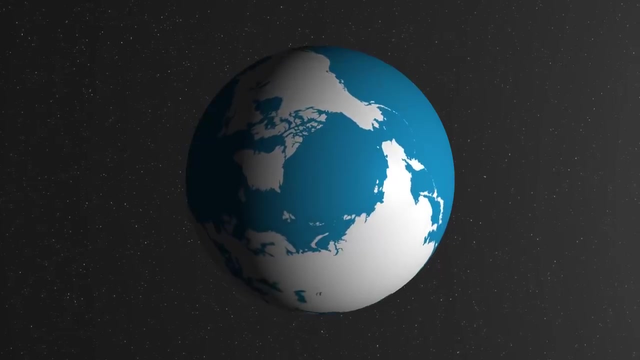 the exploitation of unconventional oils could restart with renewed vigor. This includes areas such as the Arctic, which shows promise of holding vast deposits And, with polar ice caps melting, it makes it possible to explore new areas potentially rich in oil. For more UN videos, visit wwwunorg.